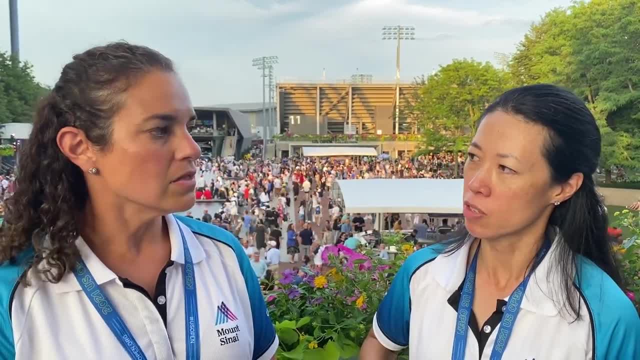 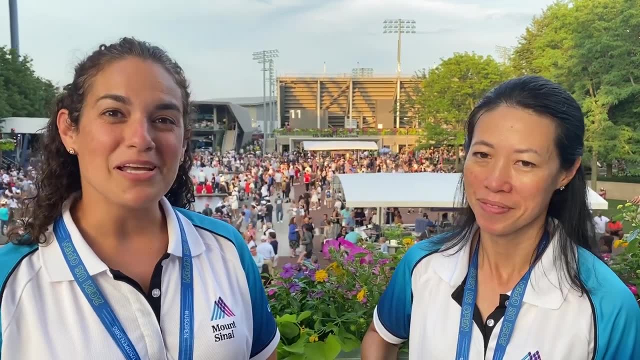 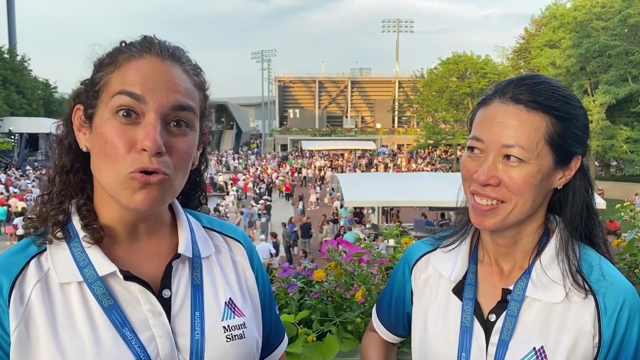 So, um, yeah, I agree with all those points. And how do you encourage your child to be a team player? Well, naturally, children grow up, I think, being very independent and not really playing well with others- like my two-year-old right now- But as they get older, they learn to interact with. 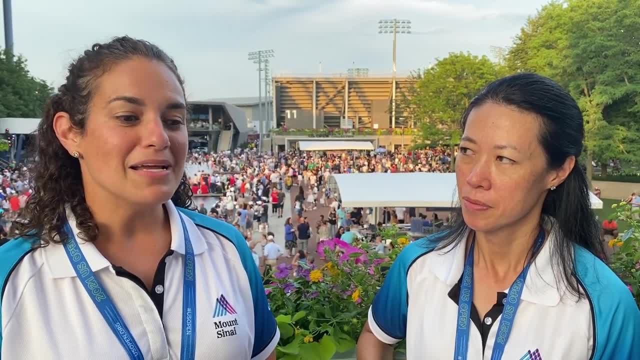 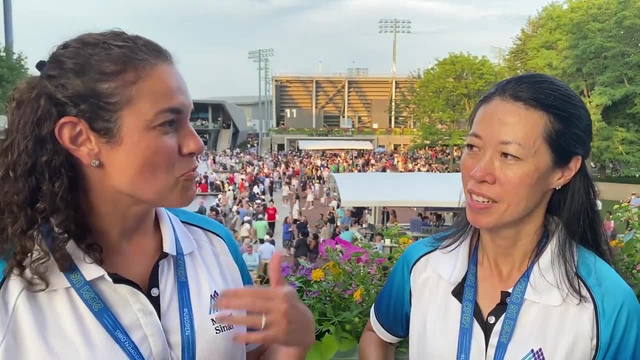 other kids and learn how to be humble and how to. it's like my five-year-old right now working on that, but, um, you know, and I know your kids are a little older, so you're probably working on different things. I think that's a really good question. I think that's a really good question. 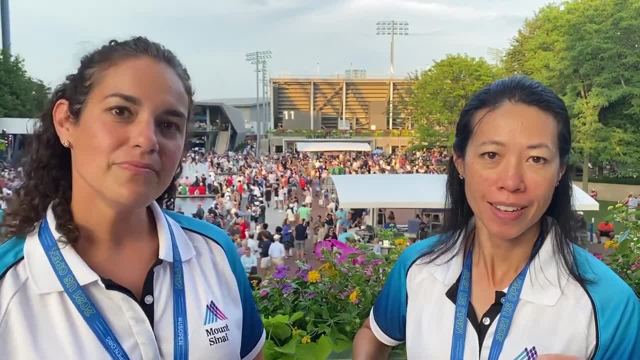 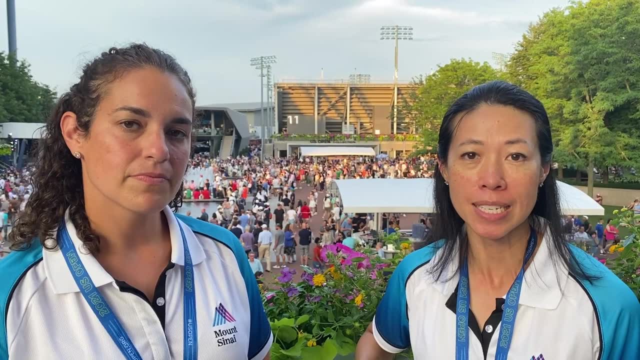 things at their level. Yeah, and I think you see it just as kids mature, that when they're younger they are more self-centered, and then as they get older, they do start to realize that there's a world around them, and and being on a team and in sports only helps them to develop that those abilities. 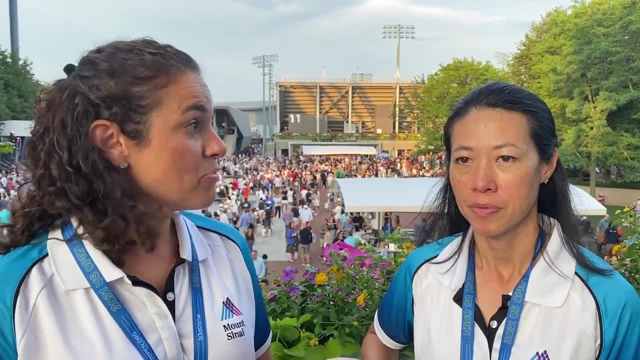 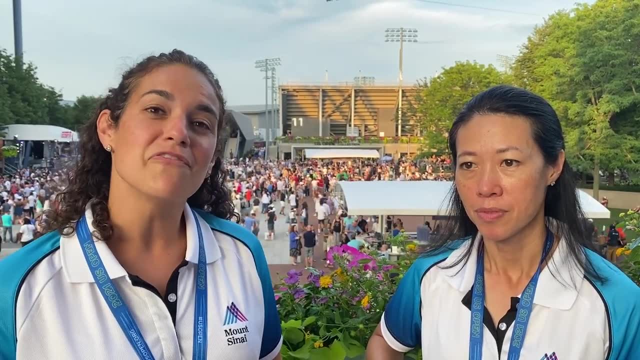 uh, to a greater extent, We also try to model that behavior in our own practice in orthopedics. We all work together um amazingly well, and we have to be a good team player, not only in sports, but also in life as well. So how can sports improve a child's self-esteem? 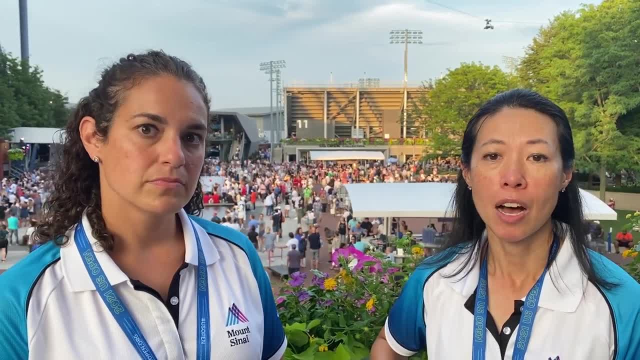 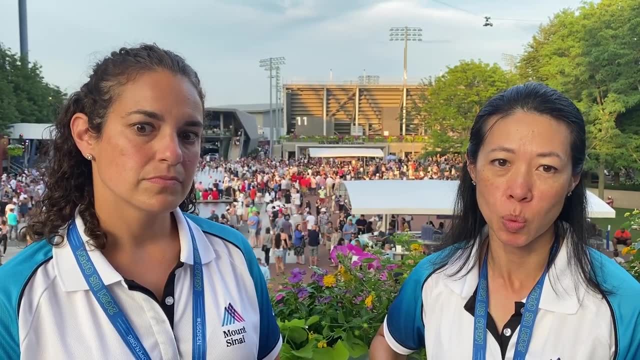 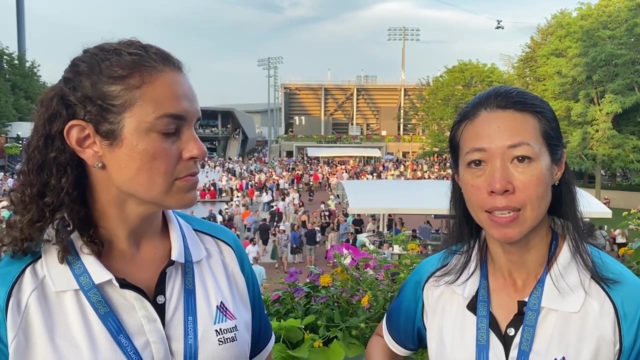 Yeah, I think that's a great question, especially because there's so much being done on grit and resilience and those sorts of things, and I think sports is definitely one of those activities where kids learn by losing and winning and being on a team, and so I think they're learning a lot of like lessons, um, in that respect. 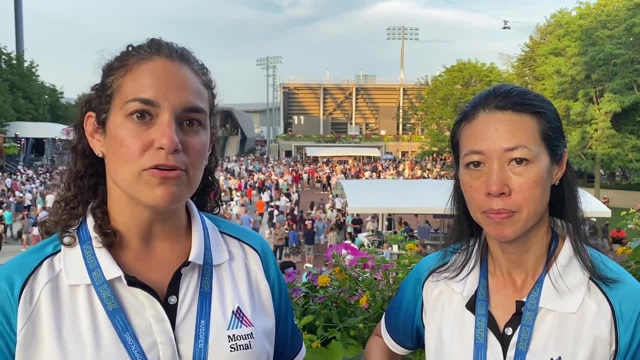 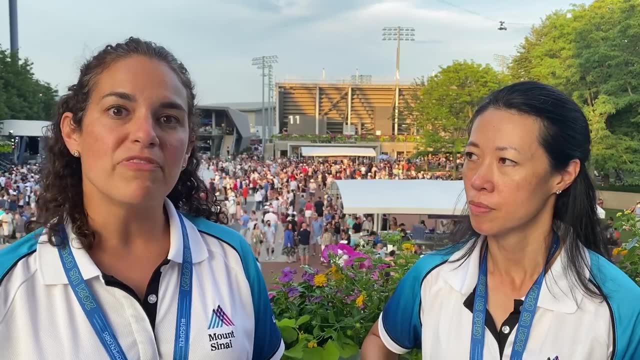 Yeah, I mean psychological stressors is a huge thing right now, especially in professional athletes as well as in children growing up with COVID and everything, and so this really provides an outlet for them to get out their aggressions but also get out some energy. Now, you don't, you want. 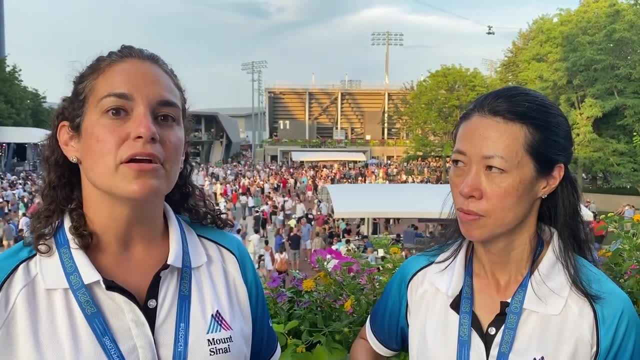 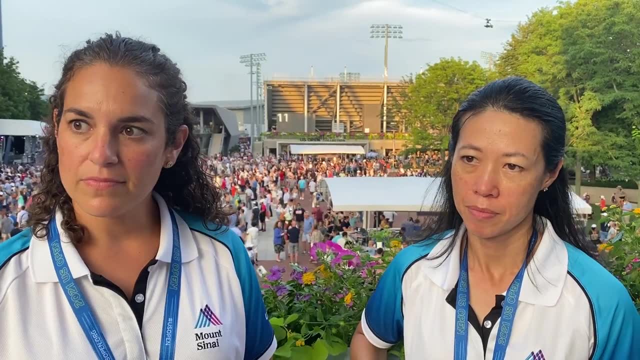 to make sure it's not creating more stress for them than they already had. but as long as they're having fun and learning what good competition is all about, then sports are great for them. So you touched upon a few things kids learn while playing sports. 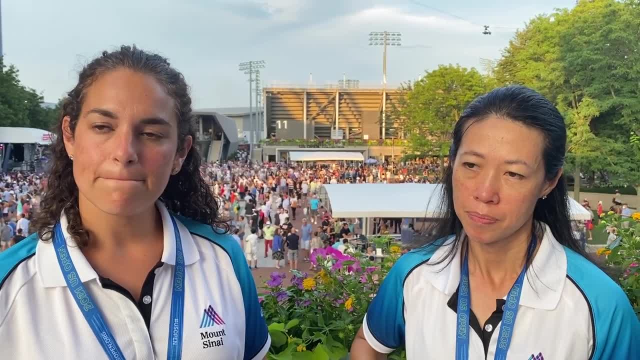 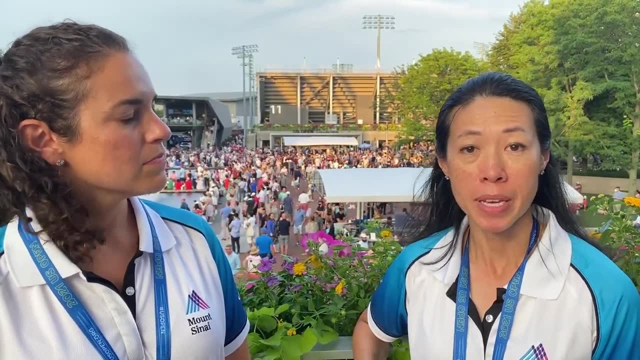 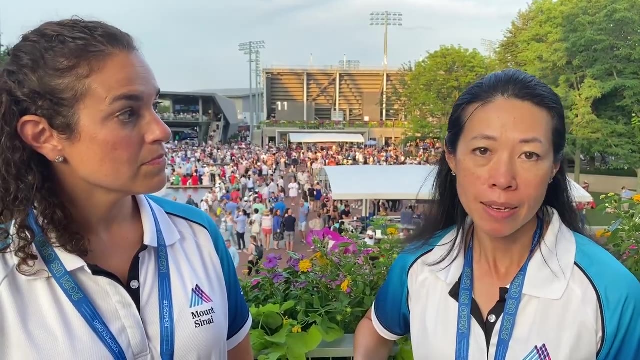 What other skills can they build on by playing a team sport? Some of the benefits of playing a team sport also translate to life itself. So cooperation, being a member or a leader or not, Always you know one role or the other, Losing as well as winning Good sportsmanship. So I think 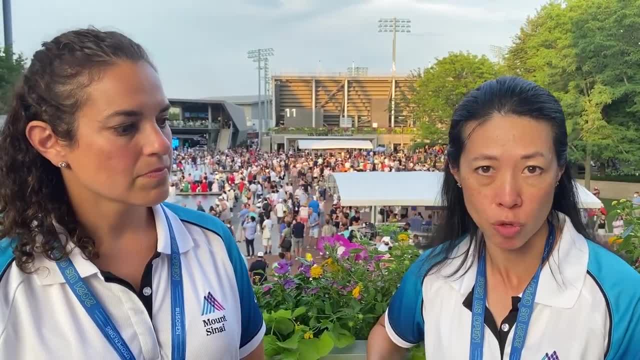 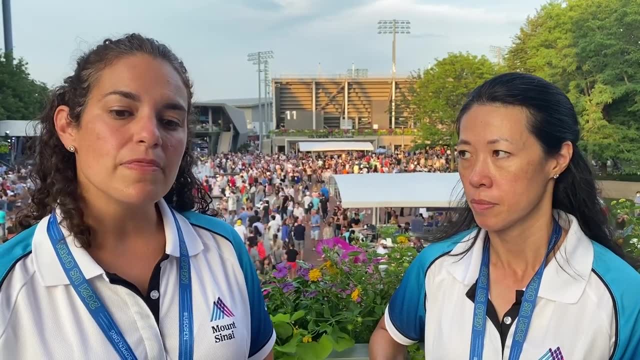 not just the athletic skills but also the life skill that then translate to being a student or then and then being in the workforce later on And you also learn. I think when you're a team athlete you learn that actually you need the entire team to win. You know, just being good yourself is not. 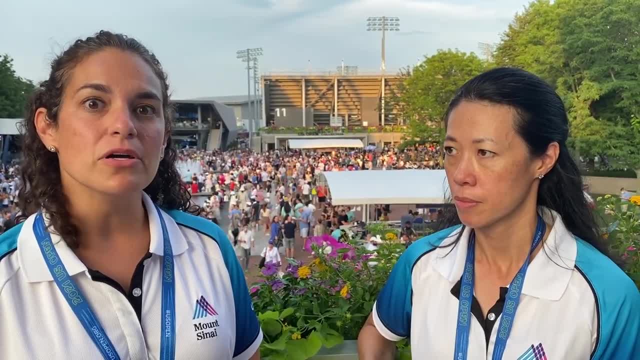 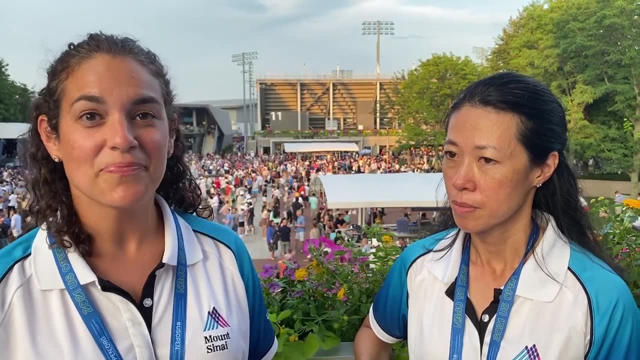 going to make or break the team. We really need everyone to be good, and so really promoting others is part of being on a team and also makes you a better person in life. I actually would also add that even if you're playing an individual sport, you do learn that. 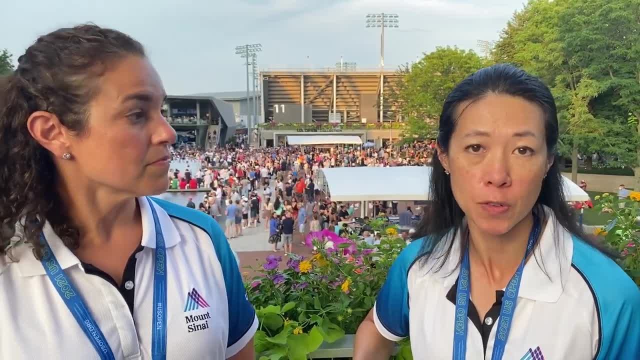 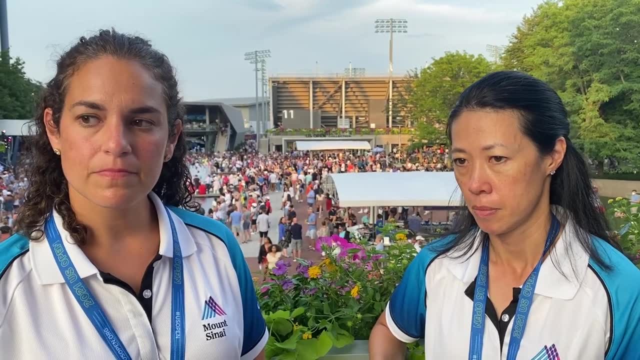 it takes a team to make you be able to win that sport or be successful in that sport. So there's very few things that we do in life where it's just the individual alone. So how do you keep your child interested or dedicated to the sport they've chosen to play? Yeah, that's oh, with the 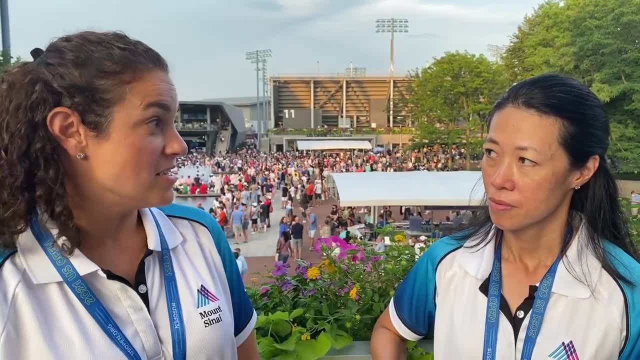 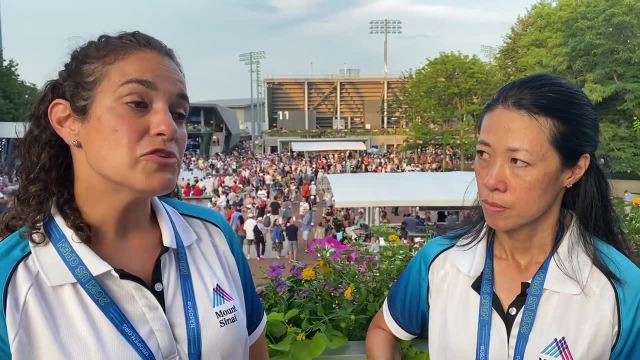 question we always actually get is whether a child should specialize at a young age or whether they can play in different sports and, you know, become good at a bunch of different sports And I think part of keeping them interested is making sure they continually love what they're. 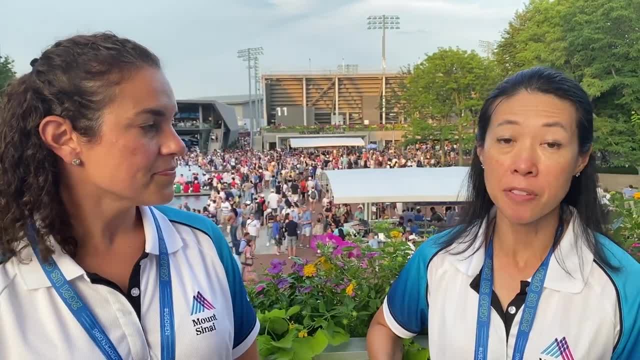 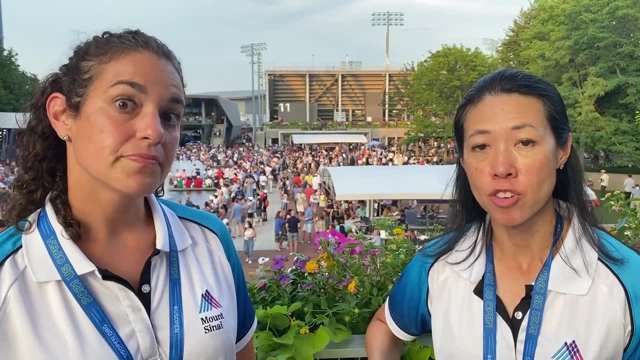 doing and it's not just all work. Yeah, I think keeping the fun in sports, I think is really important. I think on the flip side, we're both parents but we also see kids as patients in the office and there are times when we see that maybe it's not the kids idea or the kid doesn't. 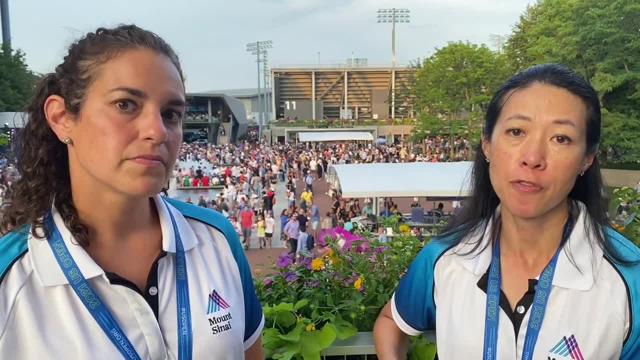 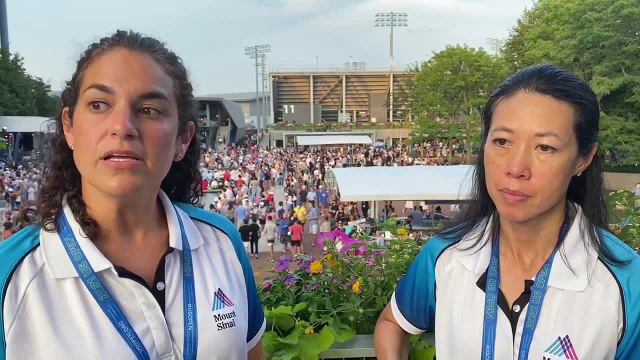 necessarily want to be participating in that activity, but it's manifesting as something else And I think having the awareness to know your child is also really important, Absolutely. So you know, either keeping them well-rounded or if they're a one-sport focus. 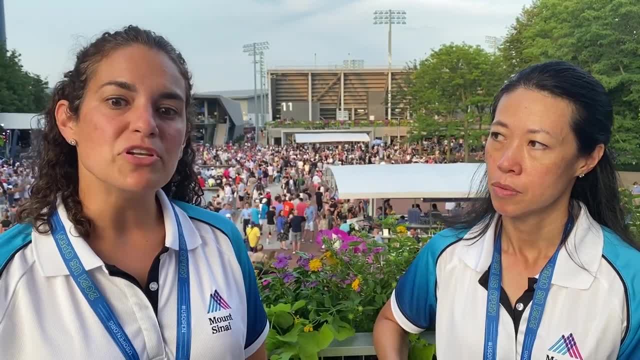 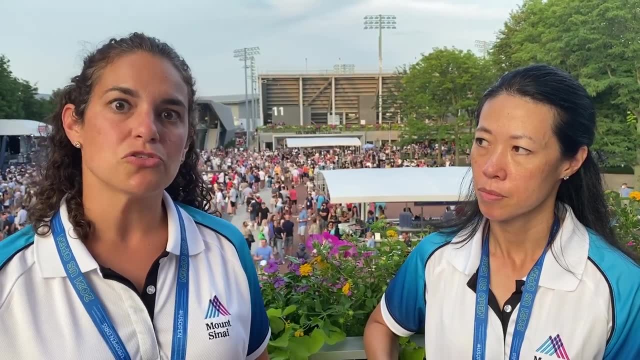 just making sure that they're always having fun and changing it up and doing other things to help that sport. So if you're a tennis athlete, obviously doing other types of cross-training that promote tennis is also really helpful so you don't get burnt out. and suffer from overuse injuries as well. Yeah, I think, both mentally and physically, it's helpful to have that cross-training, just to keep things interesting and fun and also help to improve your performance in that sport. So, lastly, how can parents teach their kids how to lose? 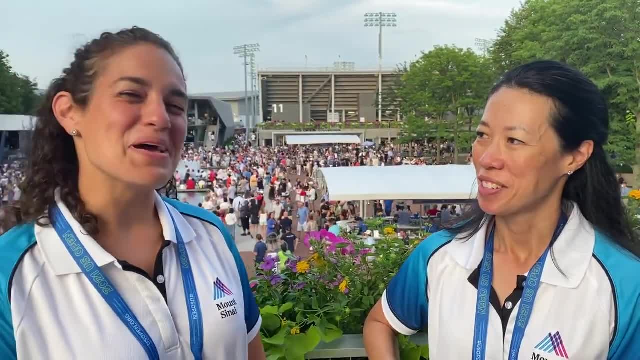 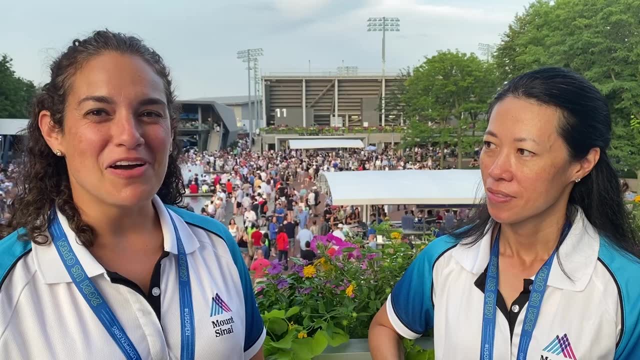 I think we're still learning that one. We're both pretty competitive ourselves And you know, I actually had a tennis match- I don't know if my partner is going to be watching this- the girl I played against, but actually the tennis match last weekend I lost.